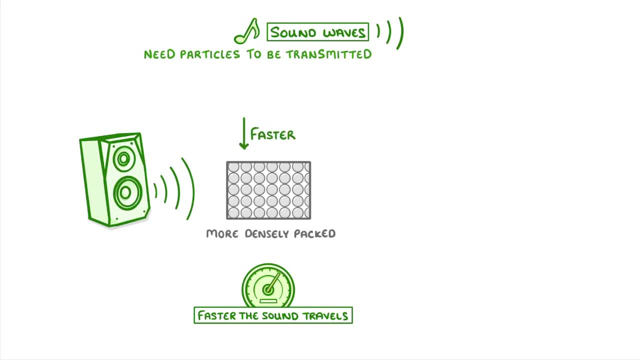 This is why sound travels faster in solids than in liquids and slowest of all in gases. It also explains why sound can't travel at all through a vacuum, Because there are literally no particles for the sound to vibrate through. Now one really important point is that as sound waves pass through the particles, they 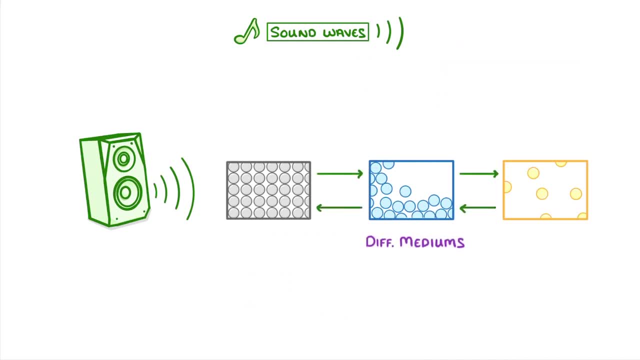 pass between different mediums and speed up or slow down, Their frequency doesn't change. The reason this is really important is because if we look at the speed equals frequency times wavelength equation, we can see that if speed is increasing but the frequency remains, the 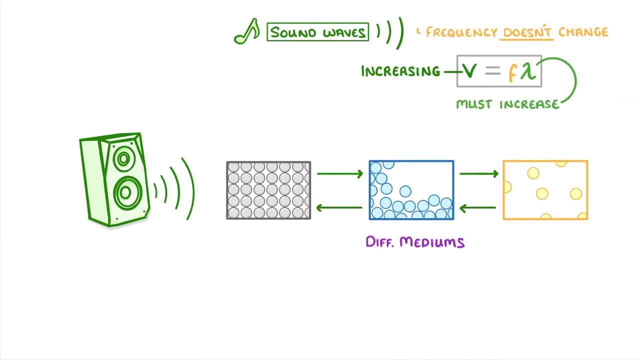 same, then the wavelength must increase instead. So the point to remember is that the wavelength gets longer, but the frequency remains the same As sound speeds up, which happens in higher density mediums like solids, whereas the wavelength will get shorter as the sound slows down in low density materials like air. 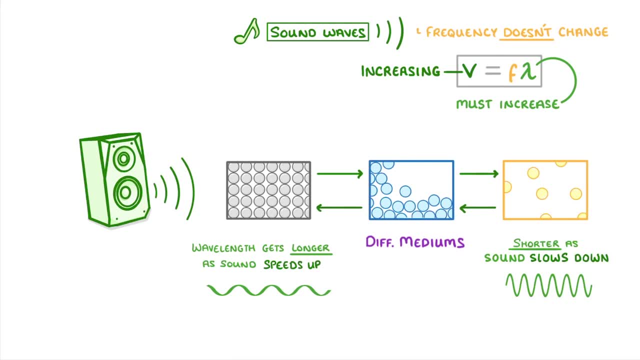 The fact that sound changes speed as it moves from one medium to another means that sound can be refracted, just like light can. Sound can also be reflected and absorbed. This is what we call a flat surface, which is what gives us echoes. 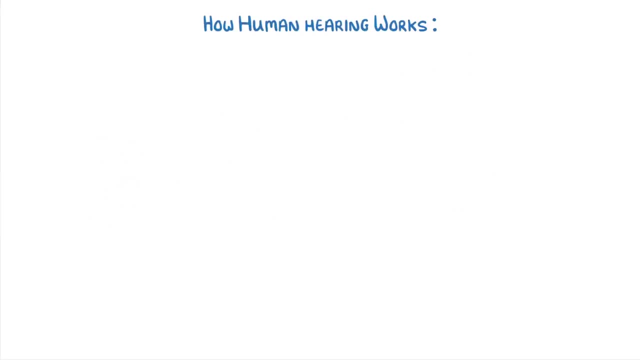 The last thing we need to cover is how human hearing works. In this picture here, we can see the entire ear. The important parts to be aware of, though, are the ear canal, the ear drum, the ossicles, the semicircular canals, the ear canal and the ear hole. 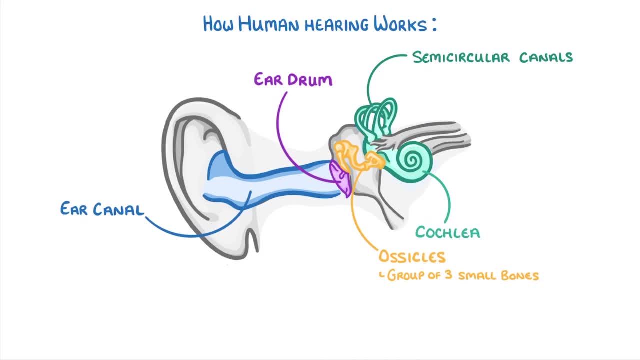 This is the ear, The ear, The cochlea And, finally, the auditory nerve. Whenever sound waves reach our ear, they travel along the ear canal and hit our ear drum, which causes it to vibrate. If we zoom in for a second, we can see that these vibrations will be transmitted along